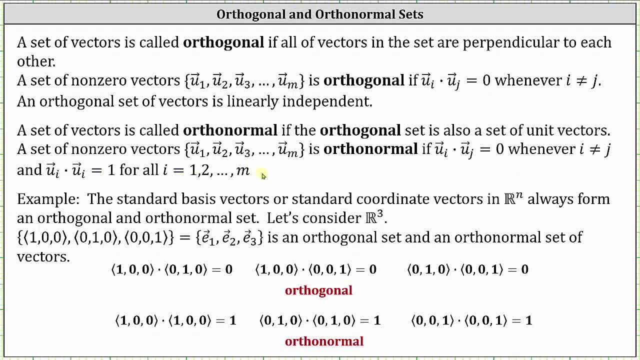 Whenever we dot a unit vector with itself, the result is always one. As an example, the standard basis vectors or standard coordinate vectors in Rn always form an orthogonal and orthonormal set. Let's consider R3, where the standard basis vectors are the vectors 1: 0 0. 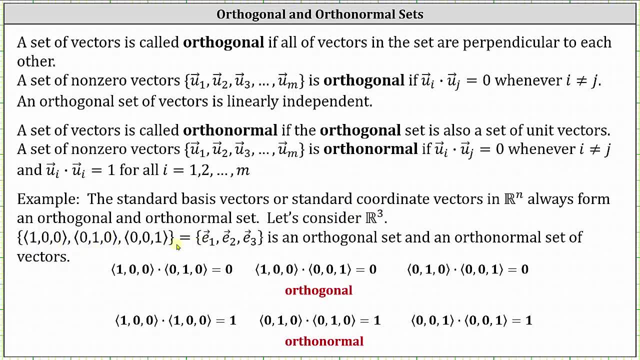 or vector e sub 1, the vector 0- 1- 0 or the vector e sub 2, and the vector 0- 0- 1 or the vector e sub 1.. This is an orthogonal set as well as an orthonormal set of vectors. 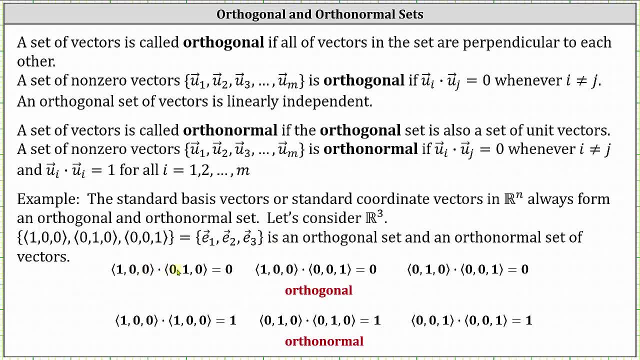 Notice how the dot product of vector e sub 1 and vector e sub 2 equals zero, as well as the dot product of vector e sub 1 and vector e sub 3, and as well as the dot product of vector e sub 2, and. 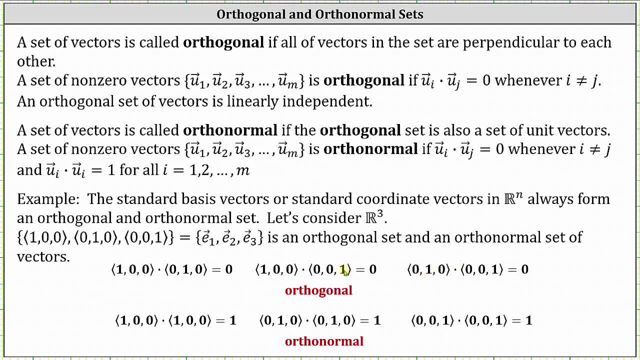 the vector e, sub 3.. So because all the dot products are equal to zero, we know the set is orthogonal And also notice how, if we take each vector in the set and dot it with itself, the result is always 0. positive 1, which indicates the set is also an orthonormal set of vectors, meaning all the 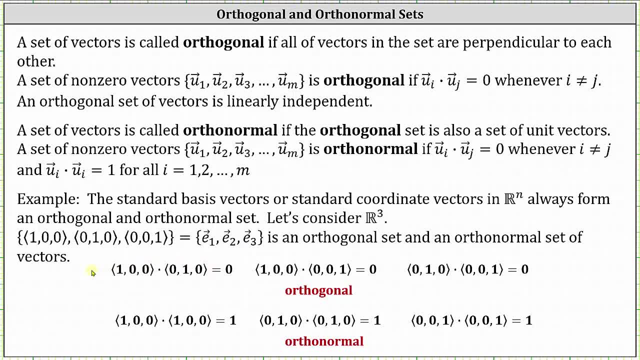 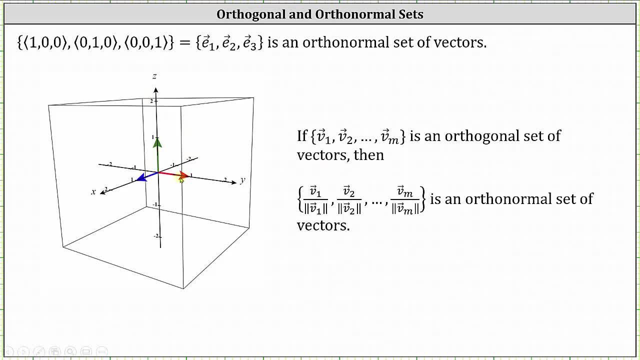 vectors are unit vectors as well as orthogonal to each other. On the left we have the graph of the standard basis vectors in R3 and we can see all the vectors are unit vectors and they are also perpendicular or orthogonal to each other. The set of vectors: v sub 1 through v sub m. 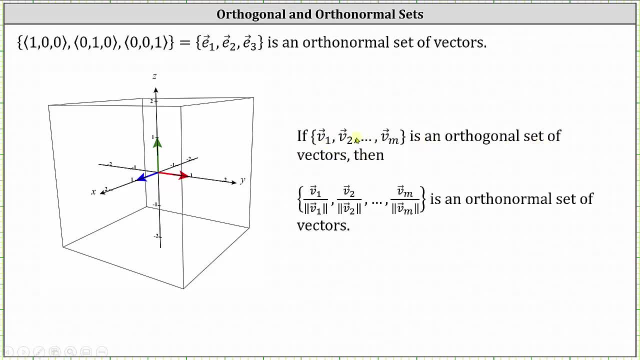 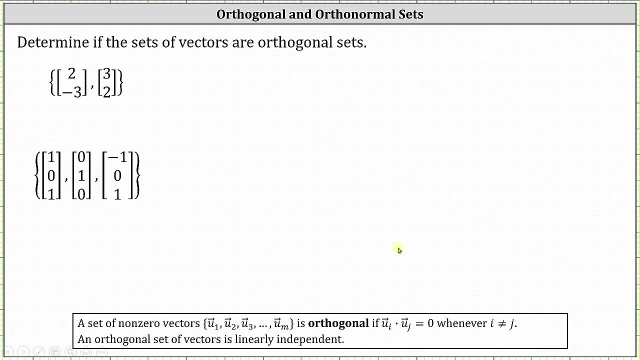 is an orthogonal set of vectors, Then if we take each of the vectors and divide by their magnitudes, forming unit vectors, the new set is an orthonormal set of vectors. Let's take a look at some examples. We're asked to determine if the sets of vectors are orthogonal. 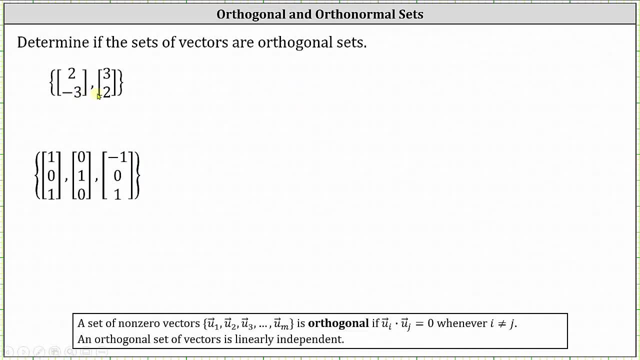 To do this, we need to check the dot products. for the first set, because we only have two vectors, We simply need to check the dot product to see if it's equal to zero. so if we call the first vector, vector u- sub 1 and the second, vector u, sub 2.. Vector u- sub 1. 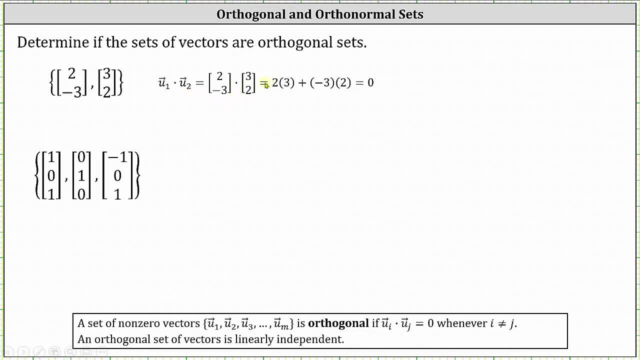 dotted with vector u sub 2 is equal to two times three plus negative three times two, which is six plus negative six, which equals zero. So because the dot product is zero, the set is an orthogonal set of vectors. In the next set we have three vectors and therefore we'll have to find vector u sub one. 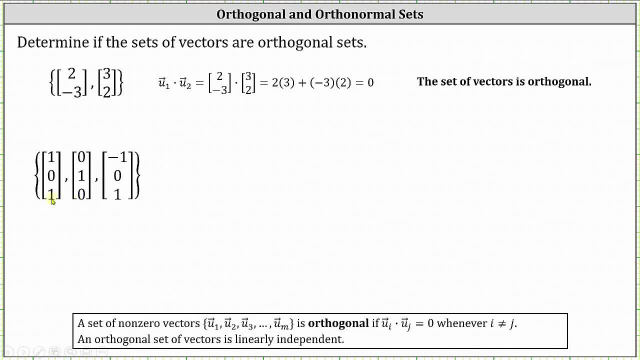 dotted with vector u sub two, vector u sub one dotted with vector u sub three, as well as vector u sub two dotted with vector u sub three. If all the dot products are zero, then the set is an orthogonal set of vectors. So let's start with vector u sub one dotted with vector u sub two. 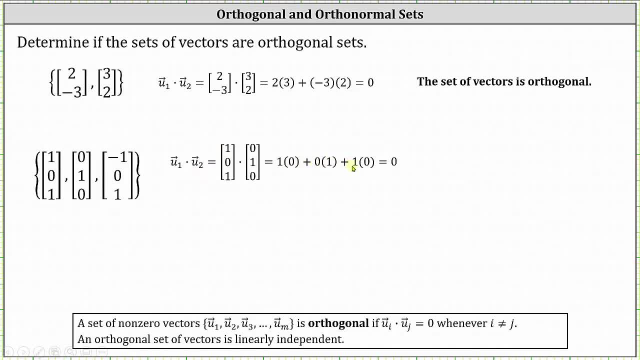 which gives us one times zero plus zero times one plus one times zero, which is zero. And now let's find the dot product of vector u, sub one and vector u, sub three, which is one times negative one plus zero times zero, plus one times one, which is negative one plus one. 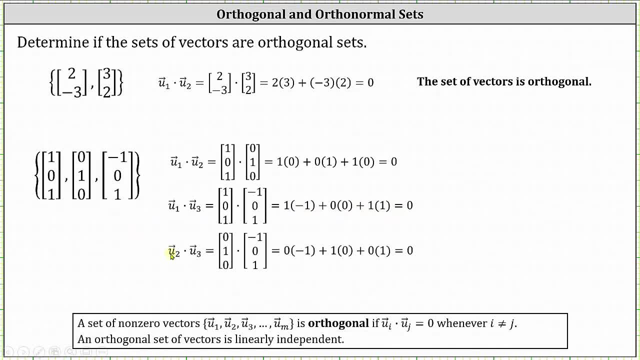 which is zero. And now let's check the dot product of vector u, sub two, and vector u sub three, which is zero times negative, one plus one times zero plus zero times one, which is also zero. So because all the dot products are zero, the set of vectors is orthogonal. 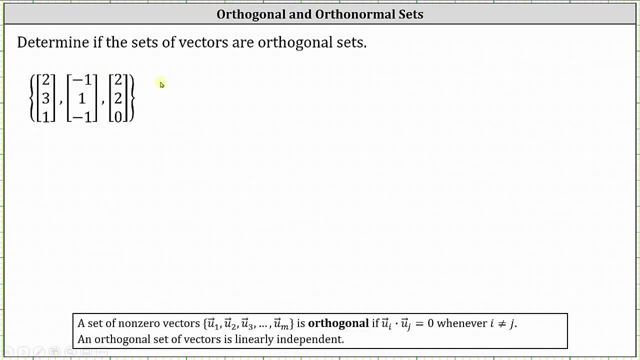 Let's take a look at one more set of vectors Again, because we have three vectors in the set, we'll have to determine three dot products Again. let's begin with vector u, sub one, dotted with vector u sub two, which is the first vector. 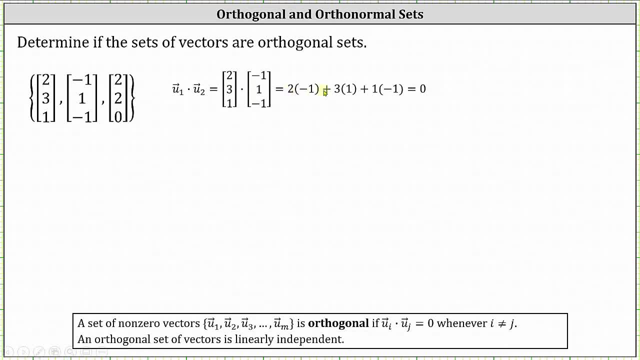 dotted with vector u, sub three. And now let's check the dot product of vector u, sub two, which is the second vector. This gives us two times negative, one plus three times one plus one times negative, one which is negative, two plus three plus negative one which is zero. 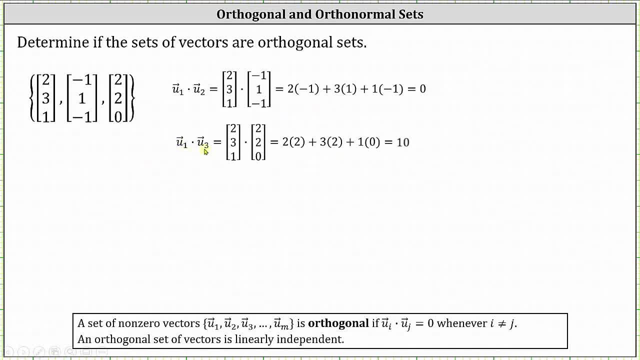 And now let's check the dot product of vector u sub one and vector u sub three, which gives us two times two plus three times two plus one times zero, which is four plus six or positive 10.. So we can stop here, because this dot product is not zero. This is not a 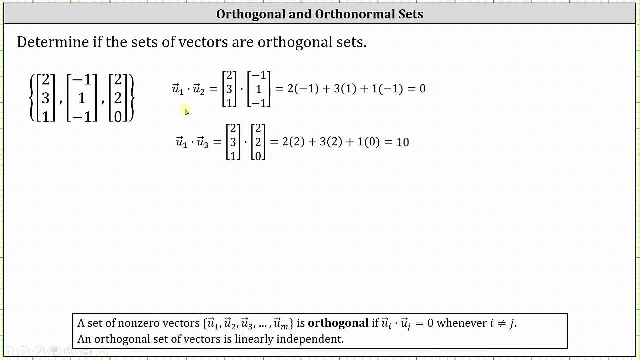 orthogonal set of vectors. But let's go ahead and just check the dot product of vector u, sub two and vector u, sub three. Notice how this dot product is zero. But again, as long as we have one dot product that's not zero, the set of vectors is not orthogonal. So again, this set is not. 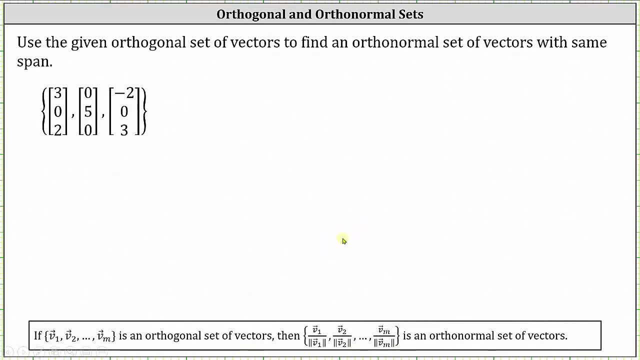 orthogonal. And then, for our last example, we are told the given set of vectors is orthogonal. We're asked to find an orthonormal set of vectors with the same span. So, even though we're told it's orthogonal, let's go ahead and check the dot products anyway. Notice how the dot products 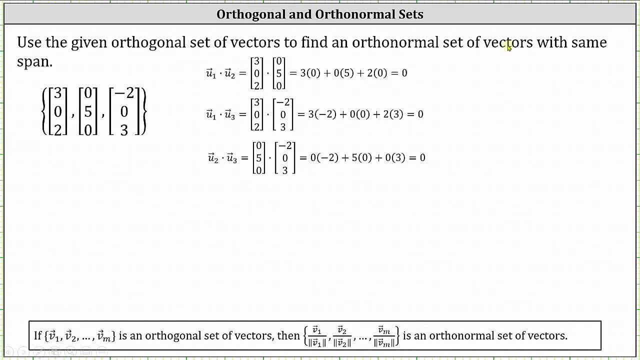 are zero. And now to find an orthonormal set of vectors with the same span, we need to find the magnitude of each of these three vectors and then divide each of the components of the vectors by the magnitude of the vector. So let's begin with the first vector, which we'll call a vector v sub. 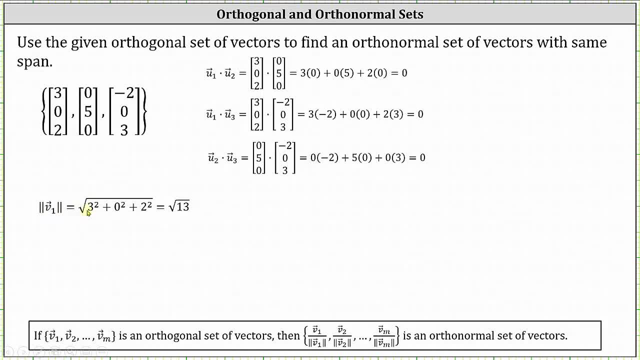 one and find the magnitude, which is equal to the square root of the sum of the square of three plus the square of zero, plus the square of two, which equals the square of three. And now let's find the magnitude of the second vector, which we'll call vector v sub two, which 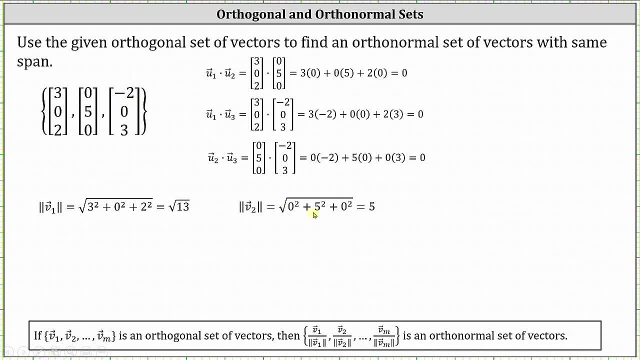 is equal to the square root of the sum of the square of zero plus the square of five plus the square of zero, which is equal to the square root of the square of five, which equals five. And then, finally, for the third vector, the magnitude is equal to the square root of the sum of the square. 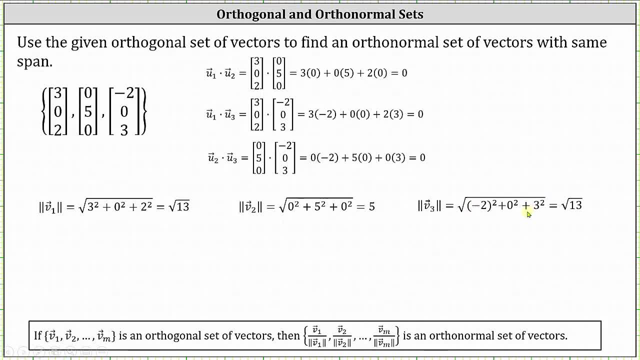 of negative, two, the square of zero and the square of three, which equals the square root of 13.. And therefore, and An orthonormal set of vectors with the same span as the given set of vectors is equal to the set shown here, where notice how we divided each component of the first vector. 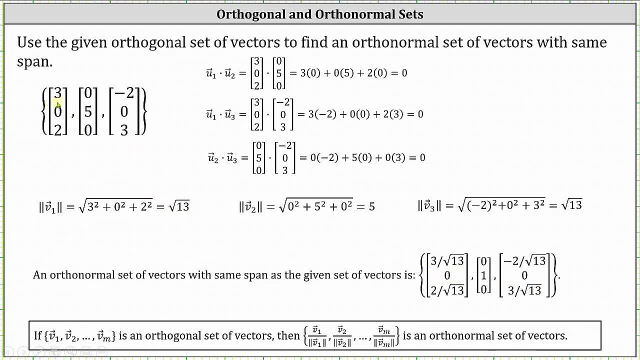 by the square root of 13.. We divided every component of the second vector by five and we divided the components of the third vector by the square root of 13.. So for this set of vectors, all the vectors are orthogonal or perpendicular, and they're.